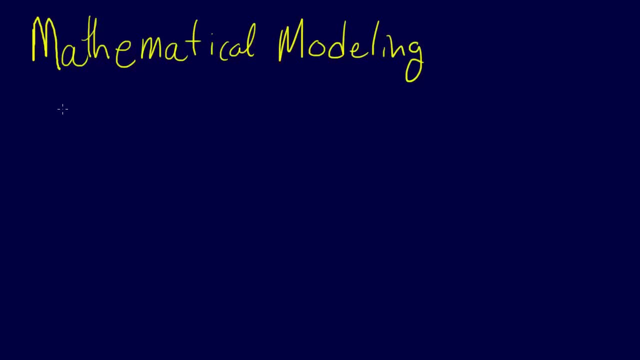 Every single one of these math problems that we've talked about. we've talked about the fact that in this course, really we're going to spend all our time learning about how to solve math problems analytically or, excuse me, numerically as opposed to analytically, which is much of what you've studied to this point. 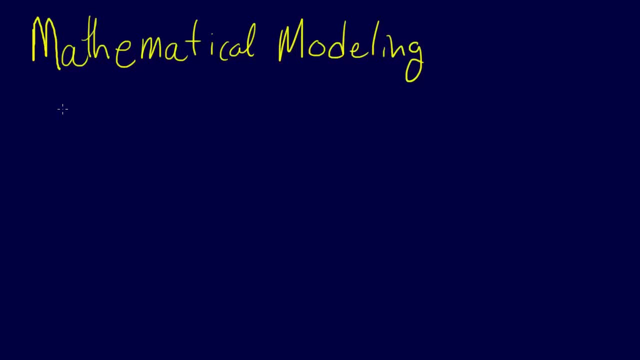 But really, before we get there, we really need to talk about where these math problems come from in the first place, And that's what mathematical modeling is all about. Every one of these problems that comes up starts with a real world problem. Okay, so there's a real world problem behind any mathematical problem that you might have. 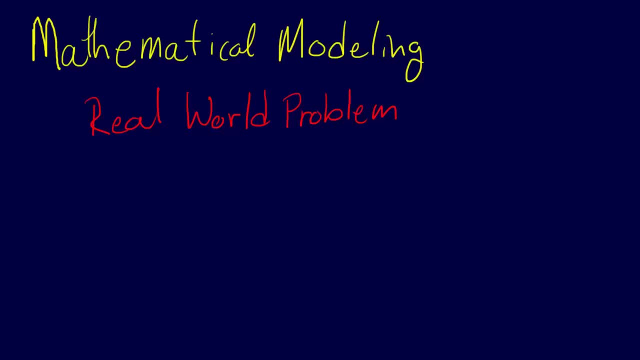 And then when you encounter, there's a real world problem. Now, that real world problem could be any problem. It could be okay. let's give some examples: It could be a problem from the financial industry, It could be a problem in transportation, It could be a problem energy. 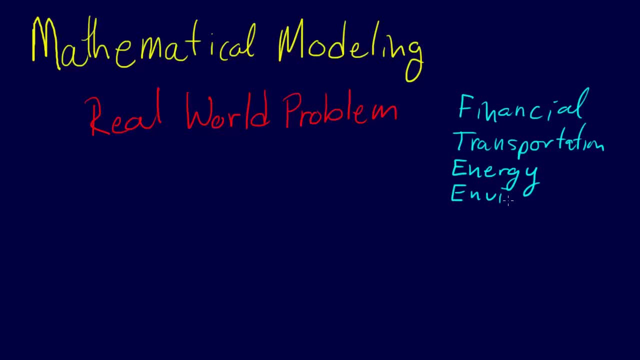 It could be an environmental problem. They are just. it could be anything. To give you a concrete example, last Christmas break I worked on this problem of it's an agricultural problem of how to do well, how to cut seed potatoes efficiently, Okay, 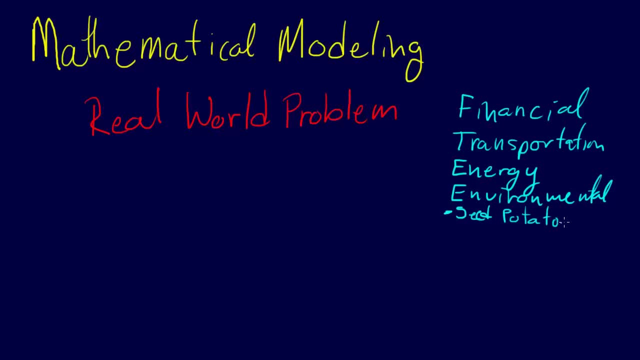 Because you have this problem of growing seeds on potatoes. Okay, there's a problem that's starting to come out of all of these There's. you have no fruit, You eat potatoes- again problem where seed potatoes have to be. if you cut them too small, then you get a seed. that's not viable. it won't grow into a potato plant. If you cut them too large, then you're wasting potentially good seed, and so you have to optimize the way that you're going to cut these seed potatoes, in addition to the fact that you're not going to do it manually. 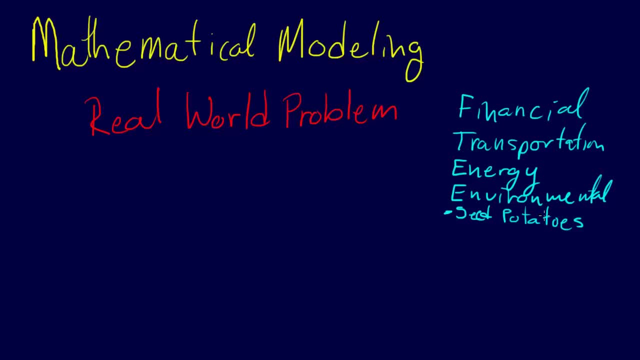 and take out a knife and cut them all up. although that's certainly possible, it's not very efficient, and so there's this complex problem with seed potatoes. That's just one concrete example where you might need to come up with a mathematical model. 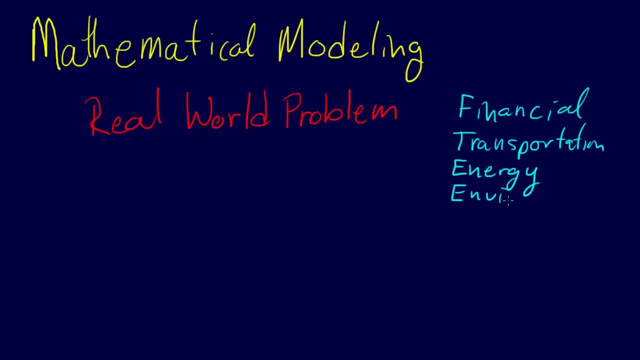 It could be an environmental problem. It could be. it could be anything, onze, There, justit could be anything. To give you a concrete example, last last Christmas break I worked on this problem. ofit's an agricultural problem of how to dohow- tohow to cut seed potatoes efficiently. okay, because you have this problem and it's sich and sand out of the shell and it's just like taking anything together and putting it in little pots and filling it in little pots of state ciao okay. okay, because you have this problem. an represents a relationship you're going to spend a lot of money on and it's good. 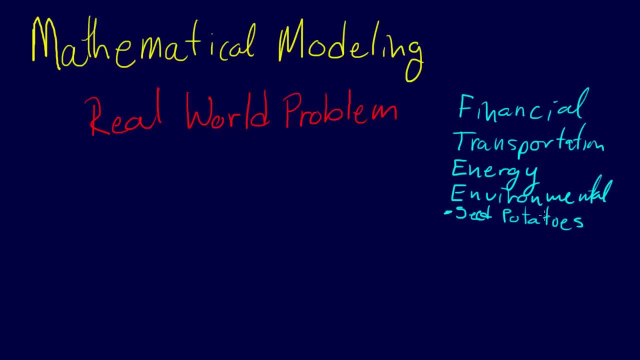 problem where seed potatoes have to be. if you cut them too small, then you get a seed that's not viable. it won't grow into a potato plant. If you cut them too large, then you're wasting potentially good seed, and so you have to optimize the way that you're going. 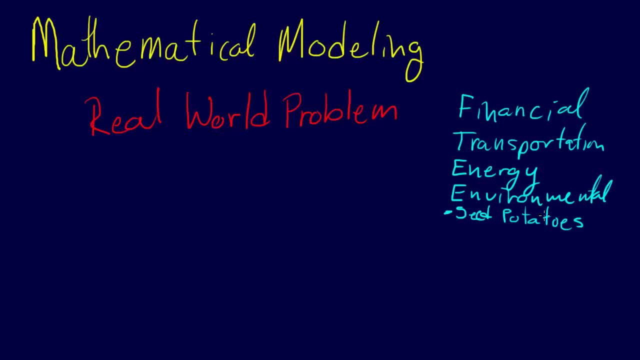 to cut these seed potatoes. in addition to the fact that you're not going to do it manually and take out a knife and cut them all up, although that's certainly possible, it's not very efficient, and so there's this complex problem with seed potatoes. That's 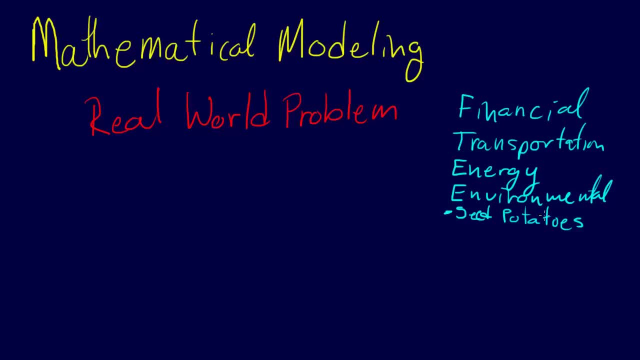 just one concrete example where you might need to come up with a mathematical model- which I actually did in this case- to address this real-world problem, and then you actually solve your mathematical, you solve the problem that you come up with. So we start with a. 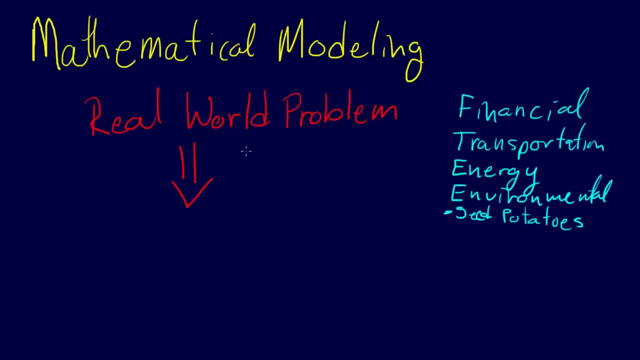 real-world problem, and then we go through this exercise, Exercise of mathematical modeling, and then we come up with this mathematical model And this whole arrow of going from a real-world problem to a mathematical model. that is mathematical modeling. And when we do mathematical modeling we have to make certain assumptions about. 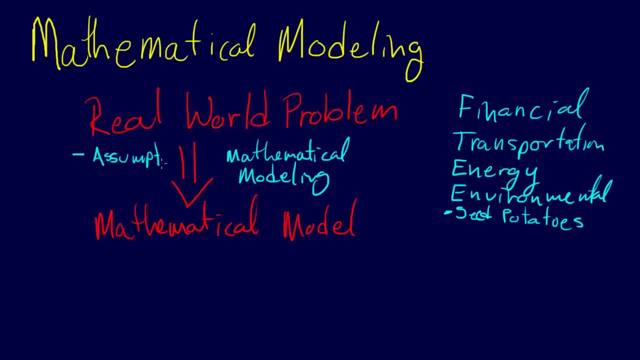 assumptions and we have to make approximations. We can just write right over the top of that. So mathematical modeling is just moving from the real-world problem to a mathematical model, by making certain assumptions and approximations but still grasping the essence of the real-world. 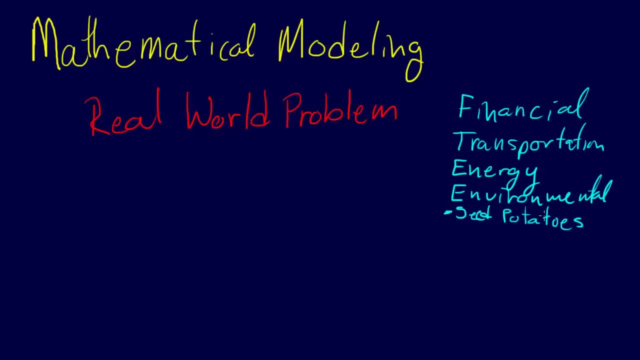 which I actually did in this case, to address this real-world problem, and then you actually solve your mathematical, you solve the problem that you come up with. So we start with a real-world problem and then we go through this exercise, Exercise of mathematical modeling, and then we come up with this mathematical model. 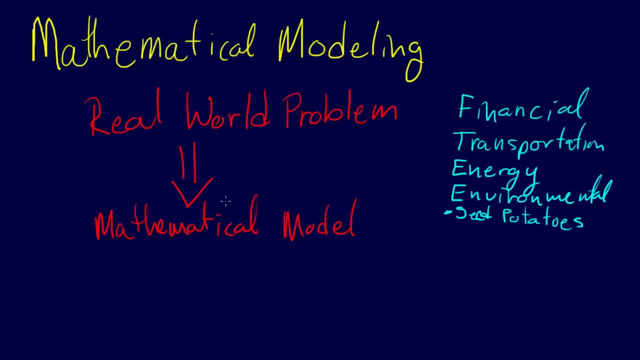 And this whole arrow of going from a real-world problem to a mathematical model. that is mathematical modeling, And when we do mathematical modeling we have to make certain assumptions about assumptions and we have to make approximations. We can just write right over the top of that. 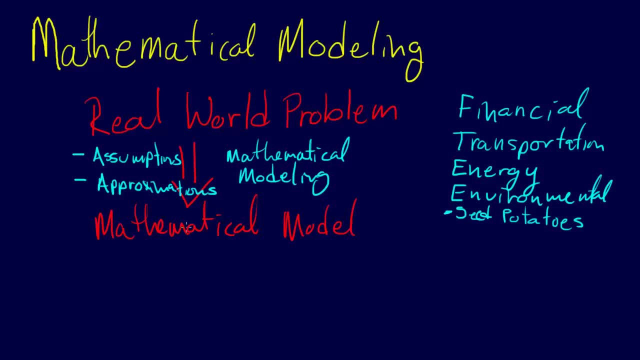 So mathematical modeling is just moving from the real-world problem to a mathematical model, by making certain assumptions and approximations, but still grasping the essence of the real-world problem. For example, we can- even we can- compare that to the definition in the textbook, which 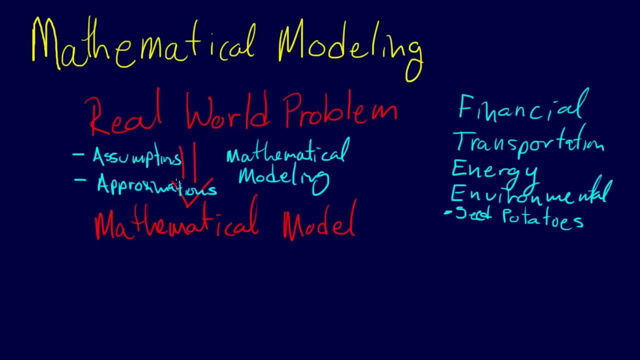 says, a mathematical model can broadly be defined as a formulation or equation that expresses the essential features of a physical system or process in mathematical terms. I just have to point out it doesn't necessarily have to be a physical system. Okay, so this is really what mathematical modeling is, and it's important because mathematical. 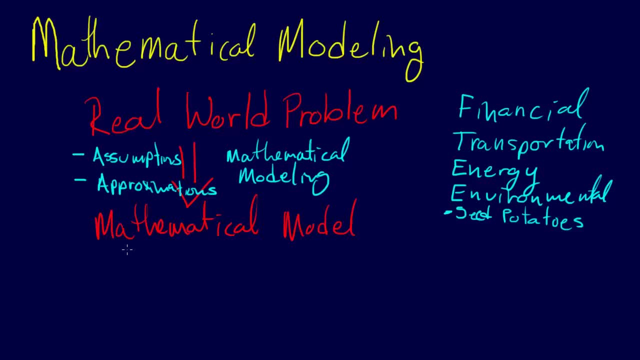 models help us understand the real-world problem. They help us solve real-world problems. We solve this mathematical model, we come up with that solution and then we apply that back to the real-world situation. And I would also point out that in this mathematical modeling step we will talk about error more in the 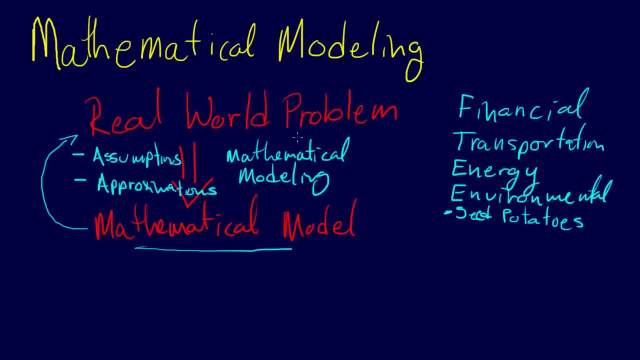 following sections. but there is already assumptions and approximations that we make when we come up with a mathematical model. In addition, when we solve the mathematical model, we'll have to make additional approximations, but as long as those approximations are close.